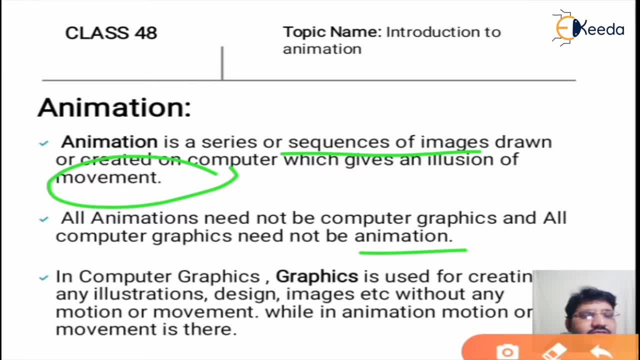 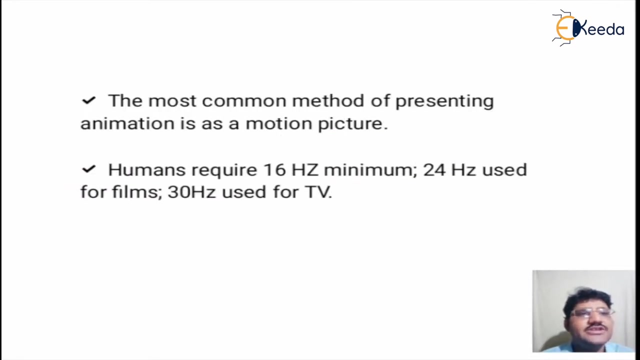 images etc. without any motion or movement, While in animation, motion or movement is there. So whenever we want to move, we want to movement in images, then we use animation. The most common method of presenting animation is a motion picture. Humans required. 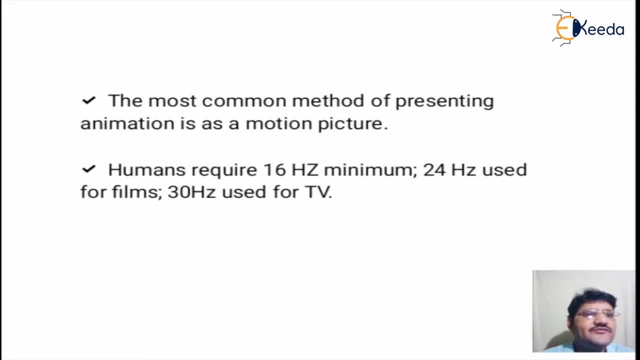 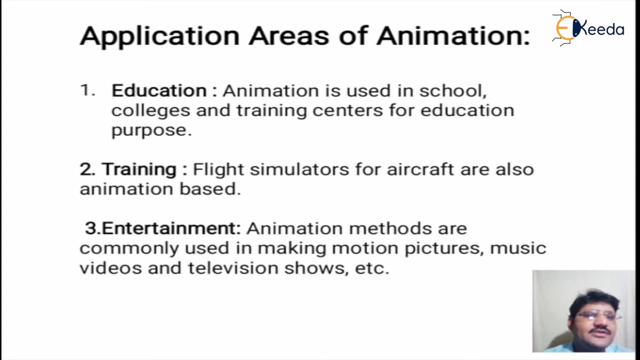 16 Hz minimum and 24 Hz is used for films and 30 Hz is used for TV for the better animation or motion of images. There are various applications where we can use animation. First, we can use animation. in education field, Animation is used. 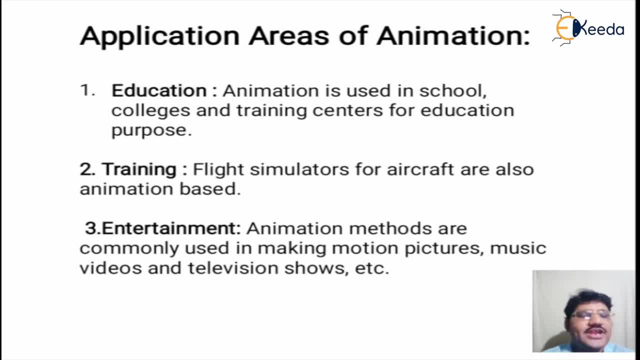 in school, colleges and training centers for education purpose. We can use animation for training purpose, like for flight simulator, for aircraft, for artifacts. we use animation For entertainment, like for pictures, movies, games, For all these. we use animation For computer aided designing. 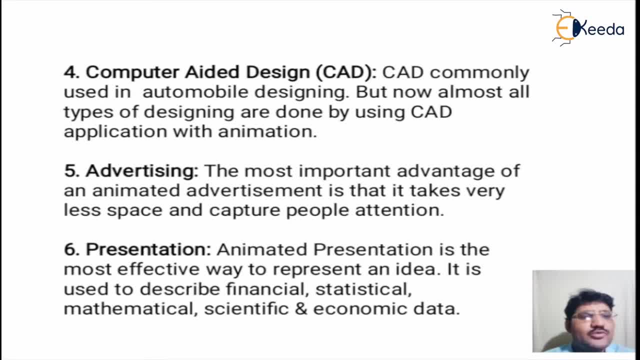 computer aided designing commonly used in automobile designing, but now a days almost all type of designing are done by using CAD, with animation In advertising. the most important advantage of animated advertisement is that it takes very less space and capture pupil attention For the presentation. animated presentation is the most effective way to 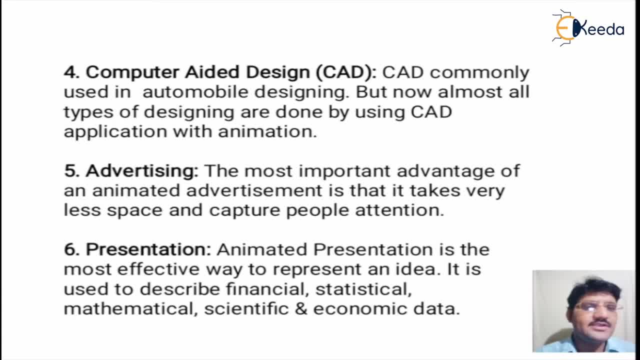 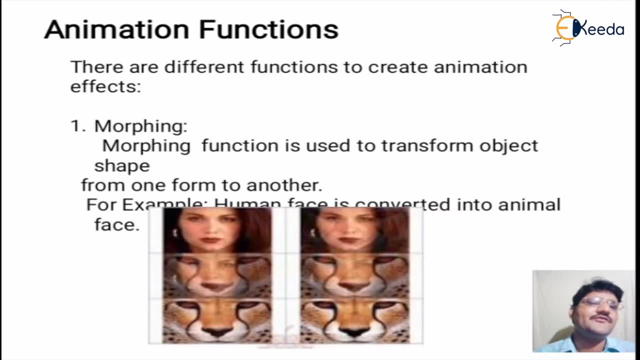 represent an idea, thought, concept. It is used to describe financial, statistical, mathematical, scientific and economic data. Now there are different functions for create animation or motion effect in an image. First is morphing: Morphing function is used to transform. 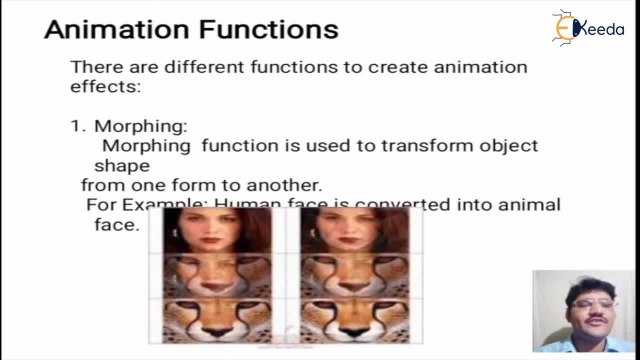 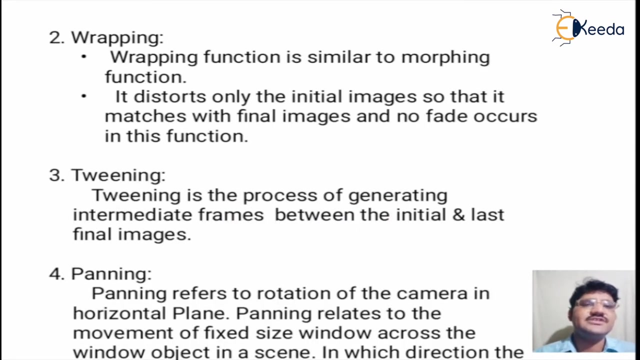 object shape from one form to another. For example in the diagram we can see here we are using morphing concept, and by morphing concept we are converting human face in animal face. So this approach is called morphing. Now, second function is wrapping. It is similar. 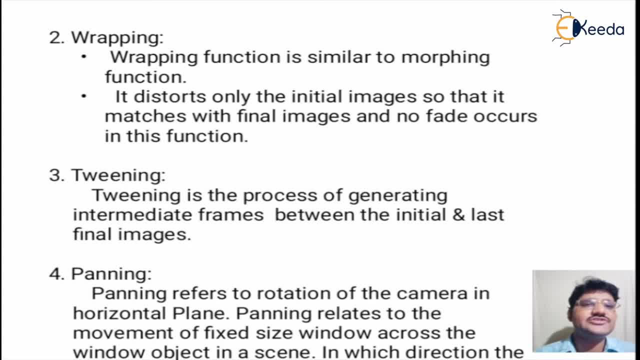 to morphing function. It distorts only the initial image so that it match with final image and no fade occurs in this function. Third is twinning. It is the process of generating intermediate frame between the initial and last final images. Next function is panning. It refers to rotation of 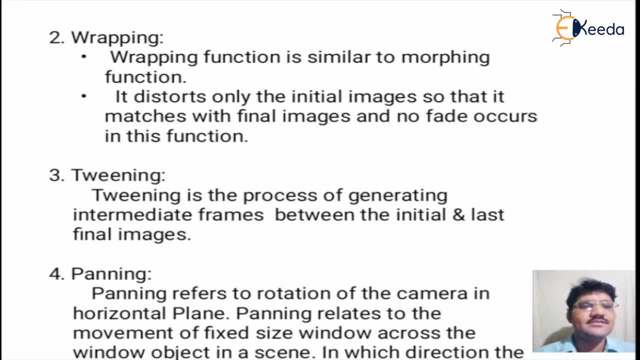 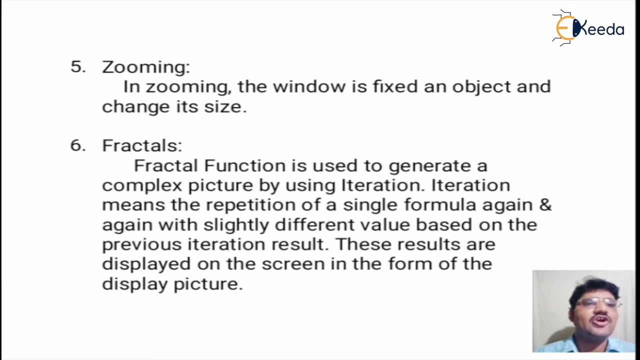 the camera in horizontal plane Panning related with the movement of fixed size window across the window object. in a scene In which direction the fixed size window moves, the object appear to in movement. Next function is zooming In. zooming, the window is fixed and object. 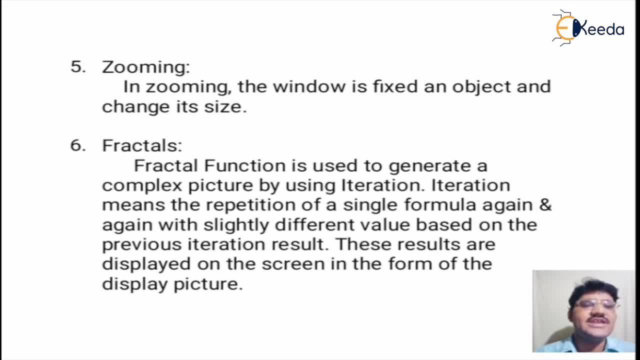 change its size. Next important function is fractals. Fractals is a very complicated pictures, Fractal images generated by using iteration. Iteration means the repetition of a single formula again and again with slightly different value based on the previous iteration result, And these result are: 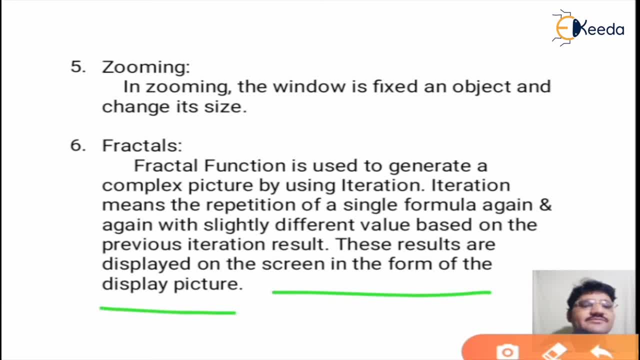 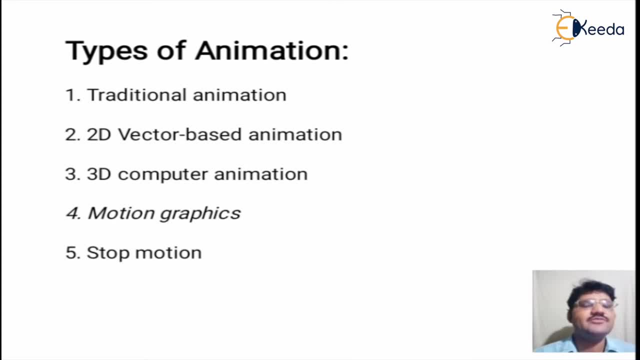 display on the screen in form of the display picture. There are different type of animation. Few important type of animations are five. First is traditional. Second is 2D vector based. Third is 3D computer animation, Fourth is motion graphics And next is stop motion. 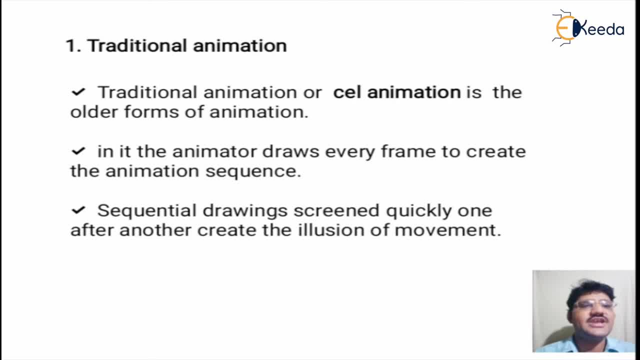 Traditional animation, which is also called cell animation. This is the oldest form of animation. Here animator draw every frame to create the animation sequence And the sequential drawing screen is designed quickly, one after another, to create the illusion of movement In second 2D vector. 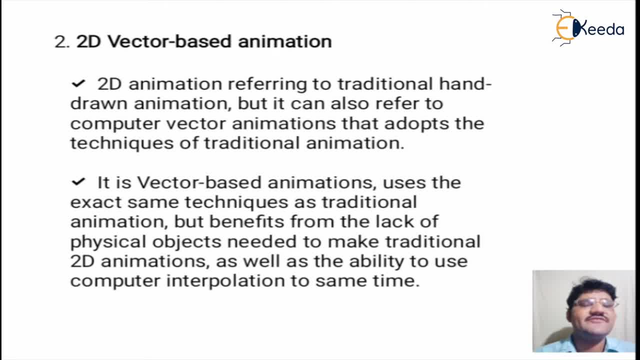 based animation, 2D animation, referring to traditional hand drawing animation, But it can also refer to computer vector animation that adopt the technique of traditional animation. It is vector based animation And it use the exact same technique as traditional animation But benefit from the lack. 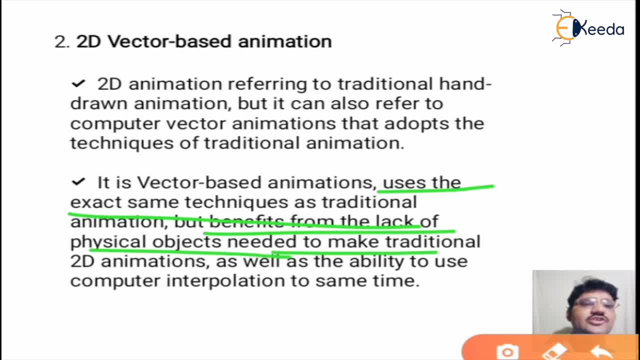 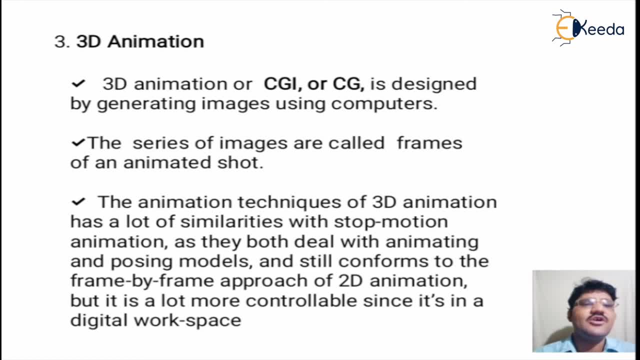 of physical object needed to make traditional 2D animation. In 3D animation, or CGI or CG, designed by generating images using computer, The series of images are called frames of an animated shot. The animation technique of 3D animation has a lot of similarities with stop motion animation. 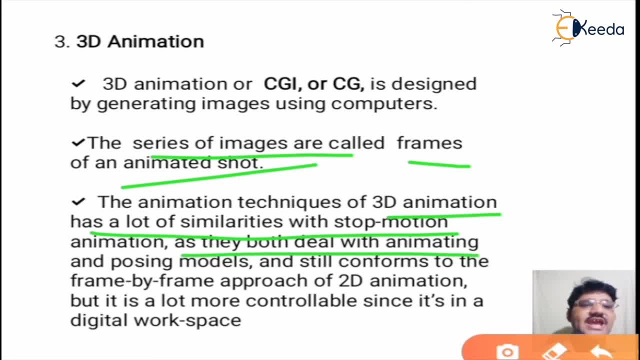 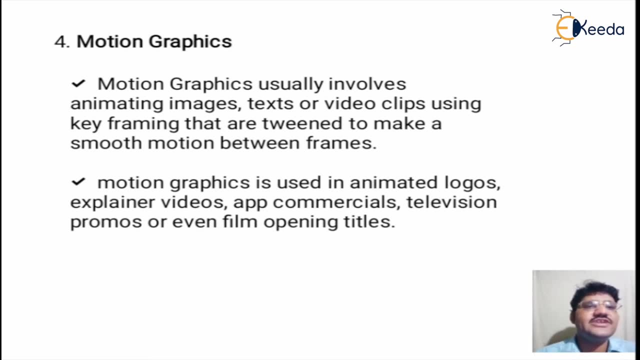 As both deal with animating and poising models And still conform to the frame by frame approach of 2D animation. In next motion graphics it usually involve animating images, text or video clip using key framing that are twined to make a smooth motion between the frames. Motion graphics: